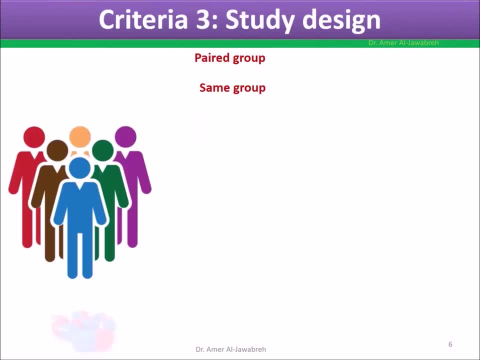 two are qualitative, while three and four are quantitative. Criteria 3: study design: Paired group, Where measurement is on the same group before and after intervention. Unpaired group, Where measurement is on two different groups. Matched group Matching is making two groups as comparable as possible by 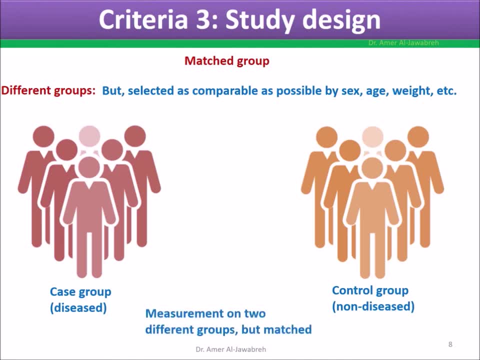 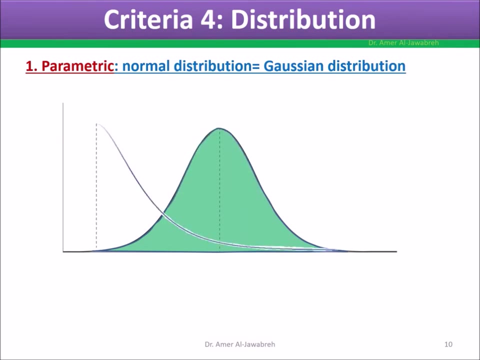 variables like sex, age, weight, etc. Measurement is on two different groups but matched. Unmatched groups: Where measurement is on two different groups that are not matched. Criteria 4: distribution. If data is parametric, like ratio data test for normality, Gaussian or non-Gaussian. If 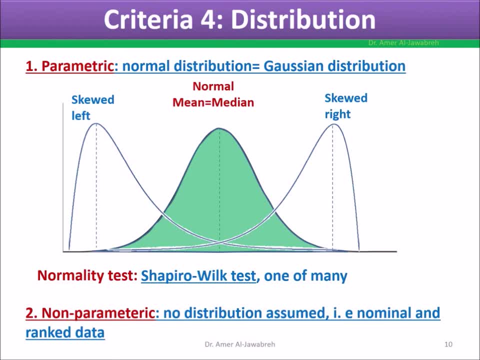 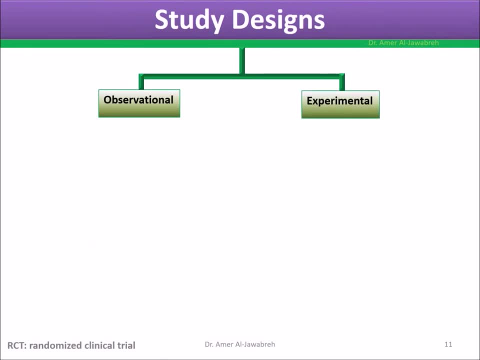 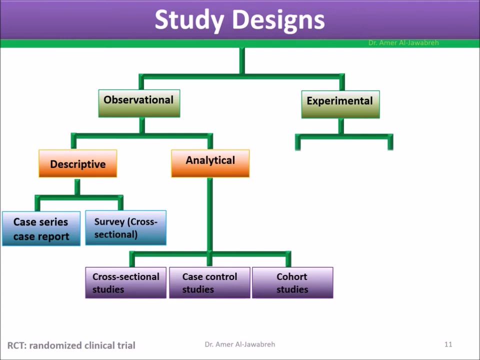 data is non-parametric, like nominal or ordinal data. no distribution is assumed. Study designs: Designs are either observational or experimental. Observational studies can be descriptive, like case series, case report or surveys. Analytical studies are either cross-sectional, case control or cohort. 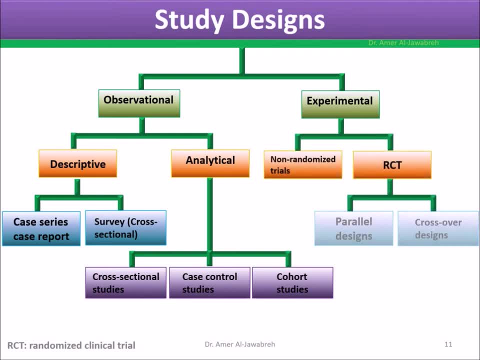 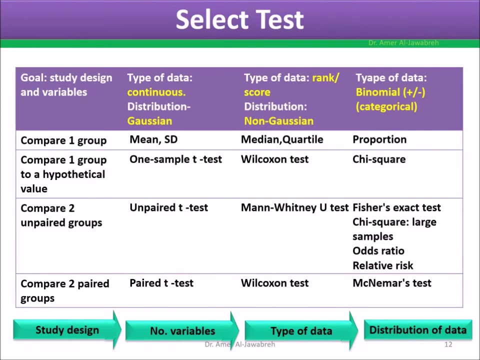 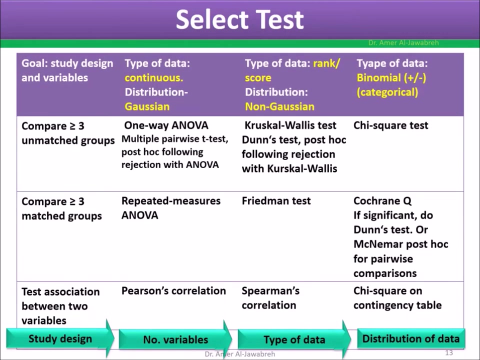 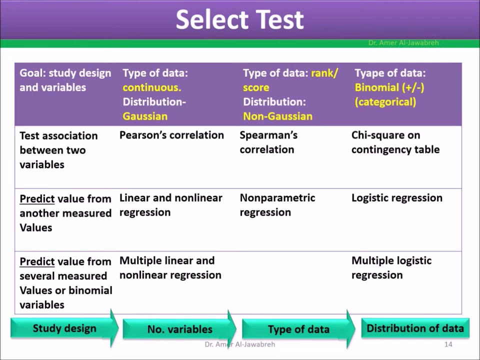 Experimental studies are either non-randomized or randomized clinical trials, which can be'm like superiority, equivalence and non-inferiority studies. Select tests: Choosing appropriate statistical tests based on the four criteria: Study design, number of variables, class and number of variables, type of data and distribution of data.